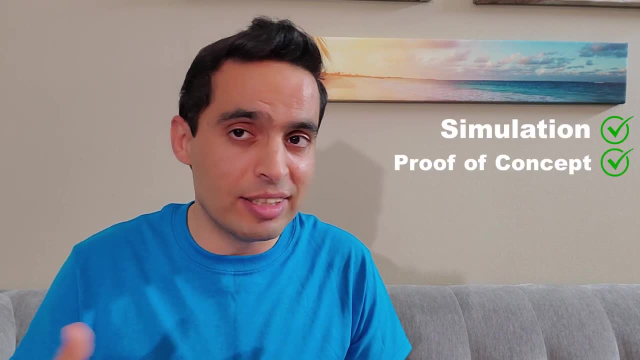 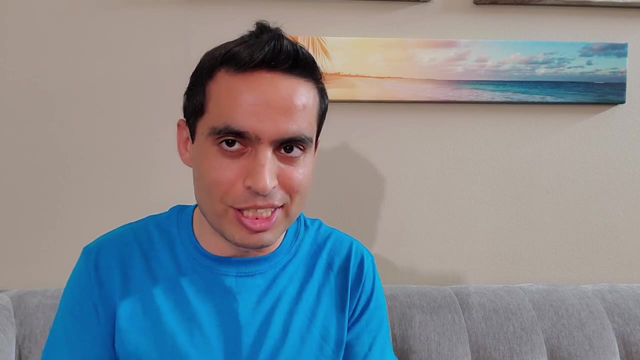 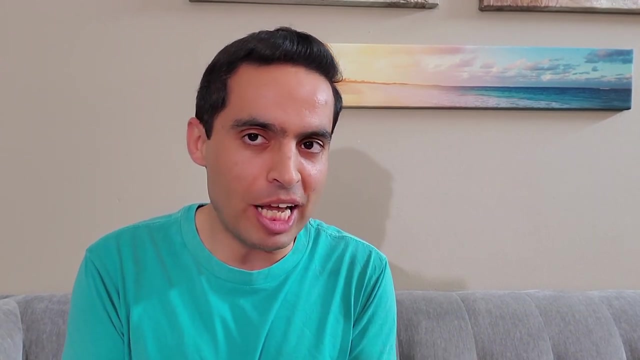 Once simulation is done, MATLAB is used in production code btcom. You just have to type your code in MATLAB��ис, and MATLAB could do a long process. Now let's talk about debate. 1. Python- Python is the second most popular programming language and the second programming language. 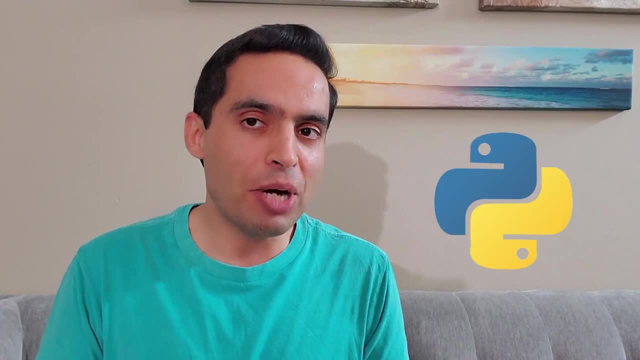 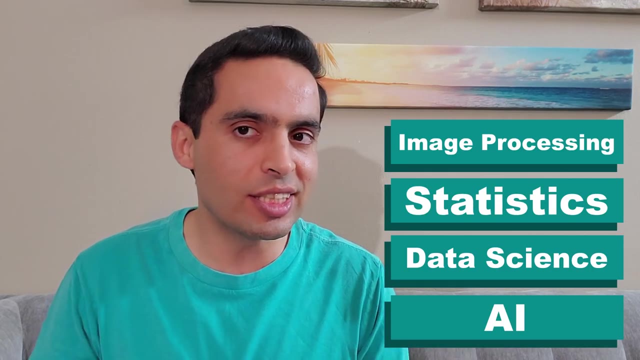 used in robotics. Here is why, Similar to MATLAB, Python comes with a ton of libraries for almost everything you can think of, from image processing to statistics, to data science and AI. It's a completely diverse and complex library. Microsoft has many libraries for a moderate number of tasks. TODAY, WE ARE GOING TO DO ANexpые. 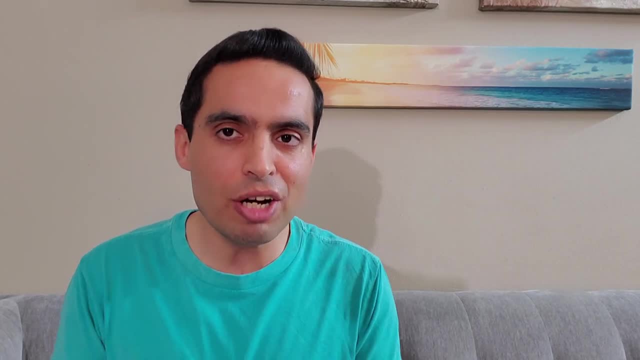 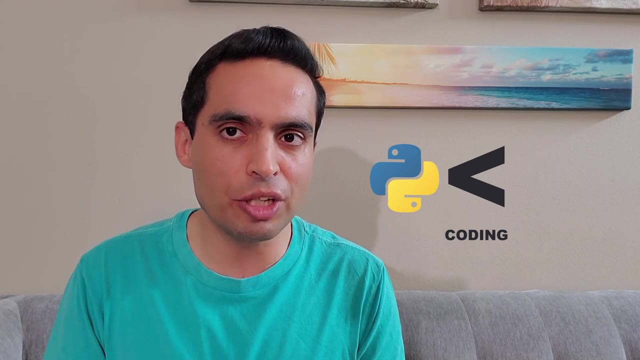 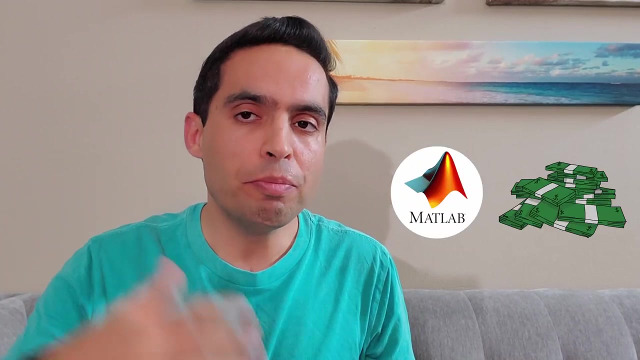 a complete package. This makes Python the king of rapid prototyping for robotics algorithm development, because much less coding is required compared to the number one language that we will soon talk about. Unlike MATLAB that you have to pay for, Python and all of its libraries are free. 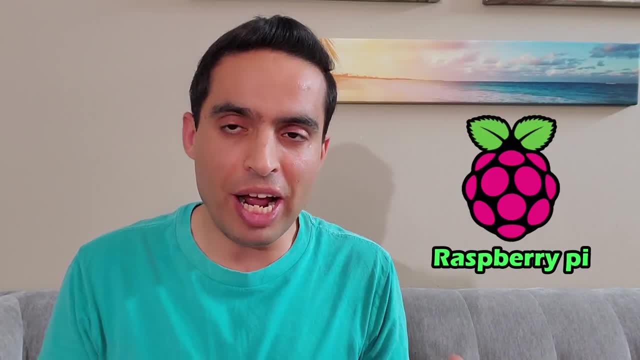 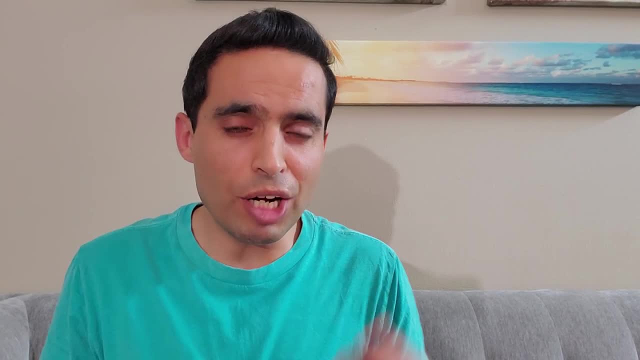 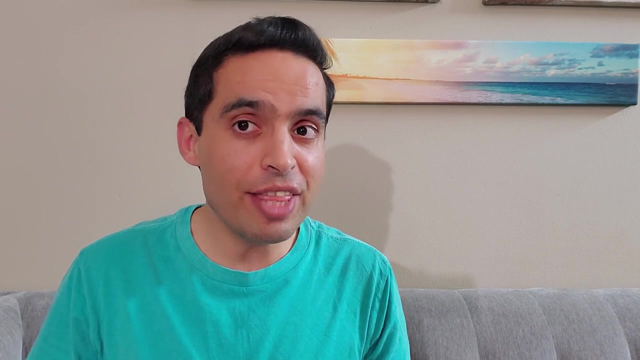 to use. Python is the primary language to program Raspberry Pi, which is a microcontroller board popular among hobbyists and students. Python is one of the two programming languages you can use in ROS, If Python used in production code. no, neither MATLAB nor Python is used in production. 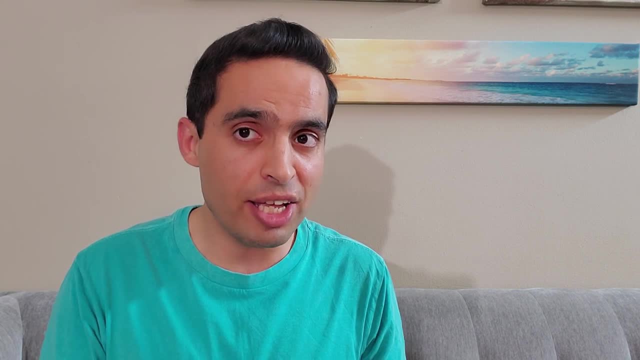 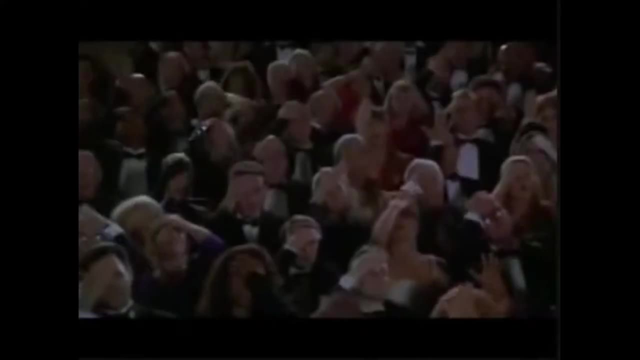 code. Once the algorithm concept is developed in Python and tested, it's translated into the number one programming language that we will talk about next. Number one: C slash C++. C slash- C++ is the number one programming language that we will talk about next. 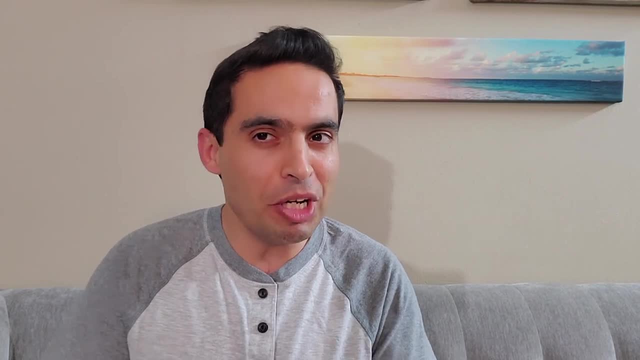 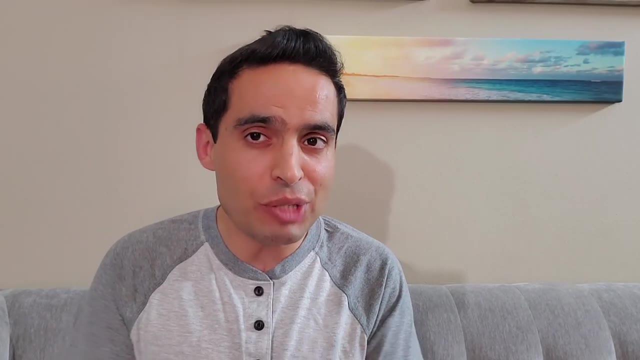 Number one programming language used in robotics. If you want to become a robotics engineer, this is the programming language you must learn. Here's why C is the language used to talk to low-level electronics. Most of hardware libraries are created in C. 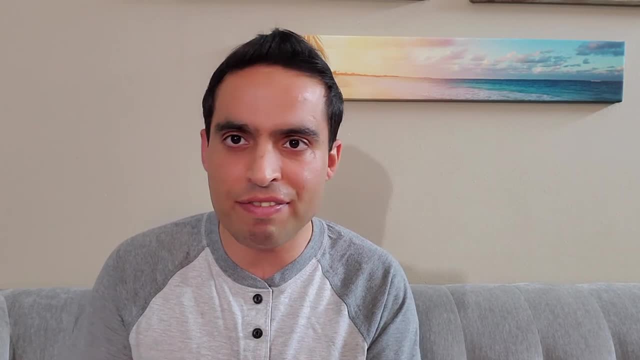 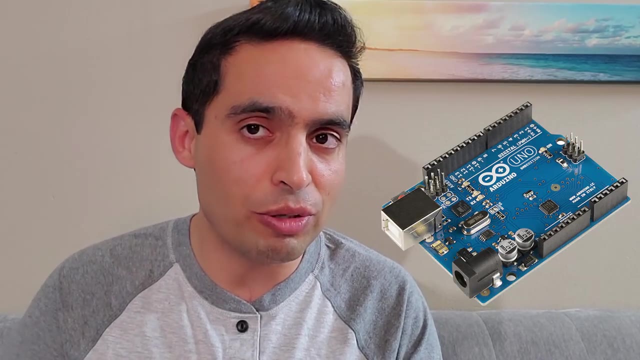 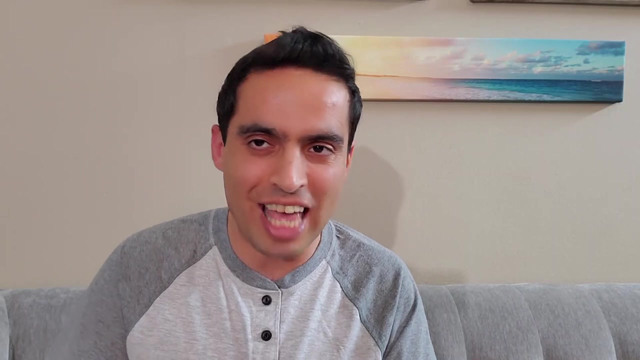 mainly because C is one of the most efficient and fastest programming languages out there. C is used to program Arduino, which is the most popular pro, The most popular pro, The most popular microcontroller board Among hobbyists and students. C++ is basically an extension of C. 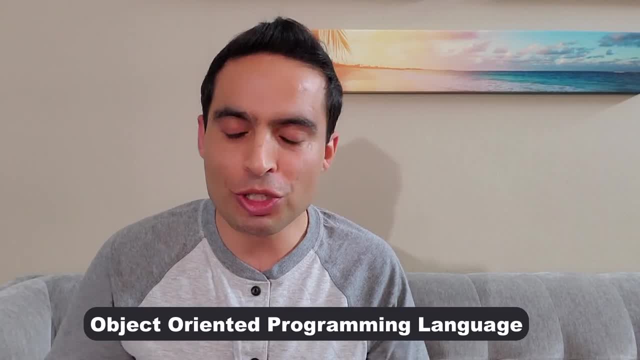 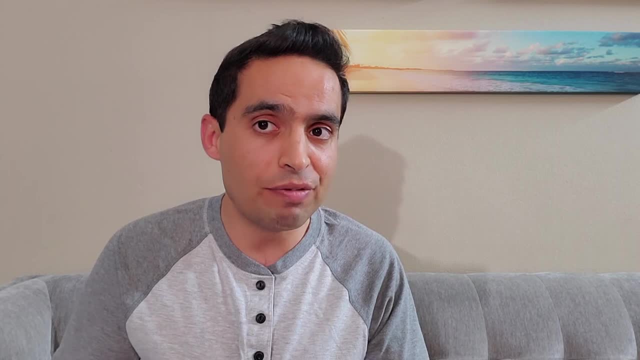 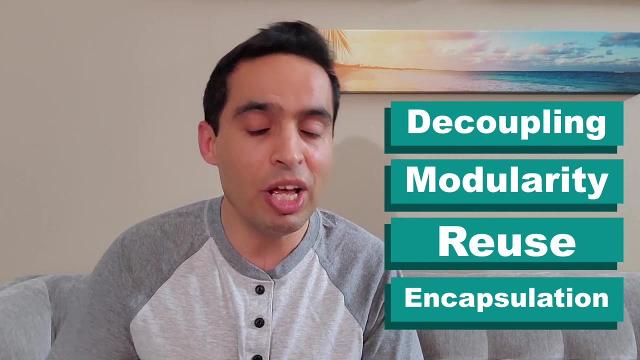 and is an object-oriented programming language, also known as OOP. OOP paradigm is used for large robotics projects because it features decoupling, modularity, reuse and encapsulation that makes large code maintainable and easy to contribute to by different developers.